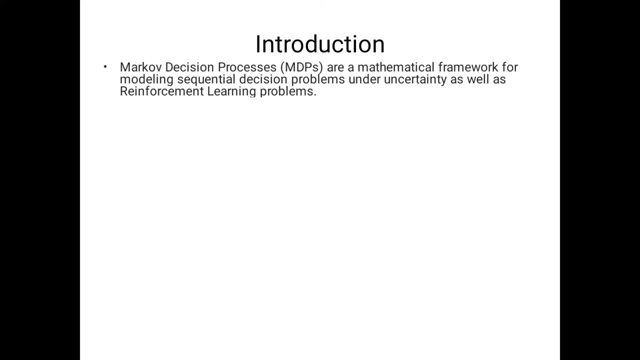 So far we have covered a lot of problem solving techniques available in the artificial intelligence, like informed searching algorithms, uninformed searching algorithms, heuristic functions, stochastic searching algorithms. But here only the difference is: here the Markov specifies the reward for who won the game. Okay, that is only the difference Maximum and all the remaining processes same for here also Okay, so actually this is a discrete time stochastic control process. 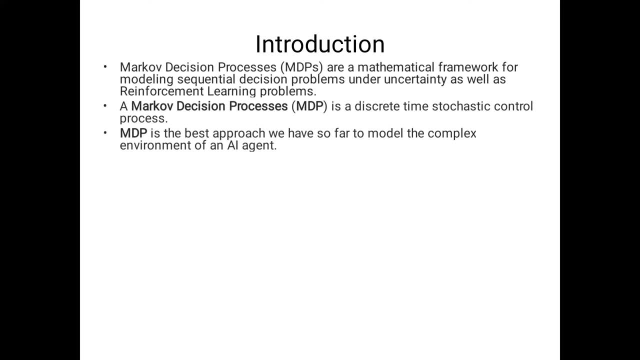 What is the meaning of stochastic? What are the examples of stochastic searching algorithms? Dice, okay, whose games are depending on the luck. Okay, so those games are related to the stochastic games. Actually, Markov decision process is the best approach we have so far to model the complex environment for the artificial intelligence agents. 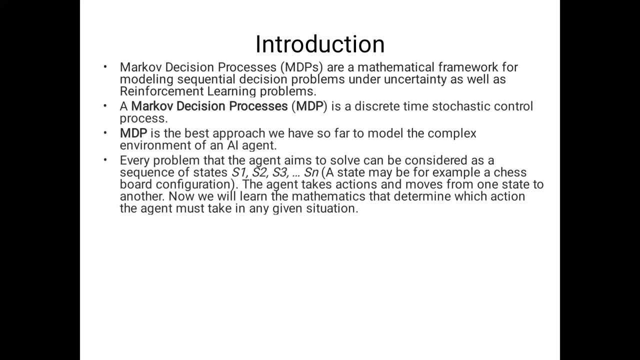 Here we have several states Already. we know how to consider the present state and present input symbol, how to find out the next state. Already we have several states Already. we have several states Already. we have several states At the time of automata theory and formal languages. here also same process we are applied. here also we will consider one state and one action. with the help of that state and action we will find out the next state. 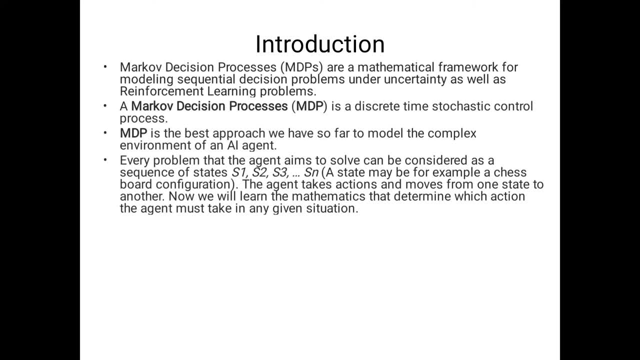 Okay, so here we will consider the sequence of states depending on the problem. So here the agent takes the actions and moves from one state to another. Okay, now we will learn the mathematics to determine which action the agent must take, Which action we choose, whether in any given situation. okay, that's why here, the markov decision process is a collection of binary ain, b, b, etc. 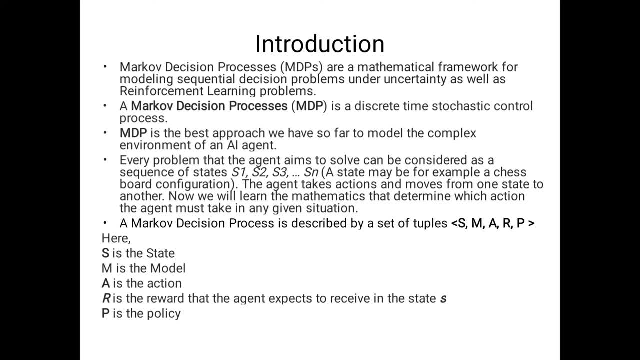 SEMARP means sequence of states. here we have. sequence of states are available. M stands for model, A stands for action, R is the reward. The special achievement in the markov decision process is the reward or reward. So the reward, the reward, is expected by the agent. 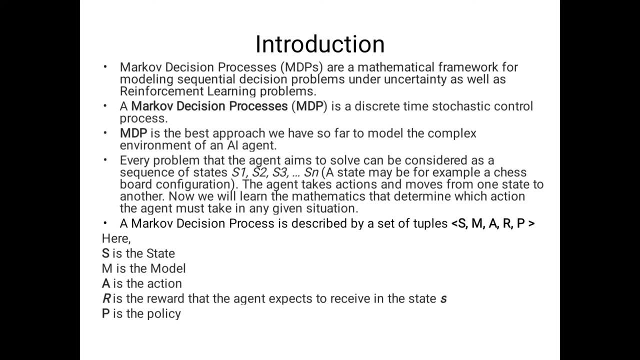 Leading the automatic decision provision on the component, with the objective of guys learning to receive in the which state. okay, so here, finally policy. here the policy means the solution of the marco decision process. now let us see what is the meaning of state, what is the meaning of model? what? 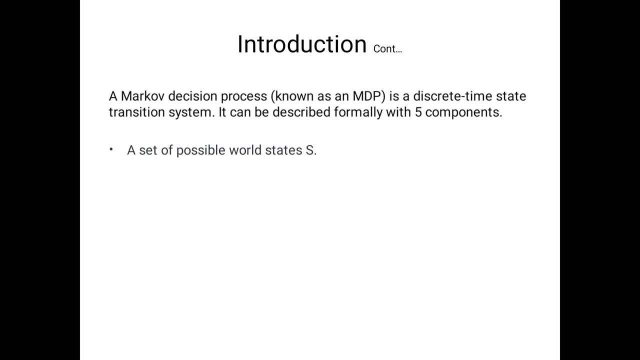 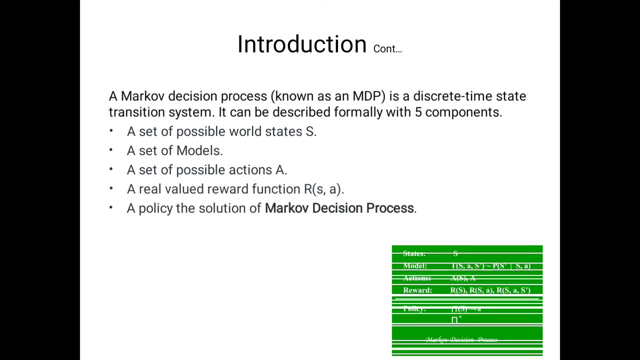 is the meaning of action, reward policy. okay, so actually this is a five components set of possible states, models, actions and reward, finally, policy. so here the states are represented with the help of capital s the model here, how the transition model is depending on the state actions and 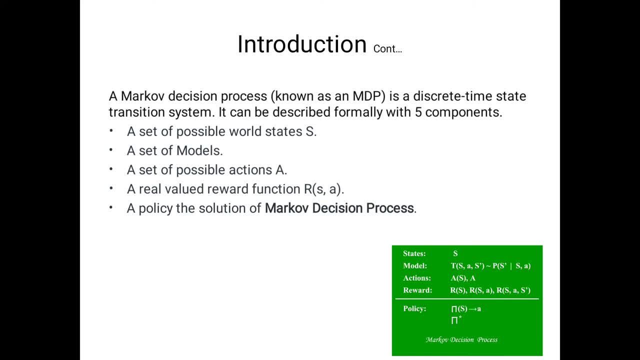 produce the solution. so that's why here t of s comma a, comma s dash. here s is the state, a is the action s dash is the next state. okay, so here the next state is dependent on the present state and the action. so here we will find out. each and at each and every step we will find out. 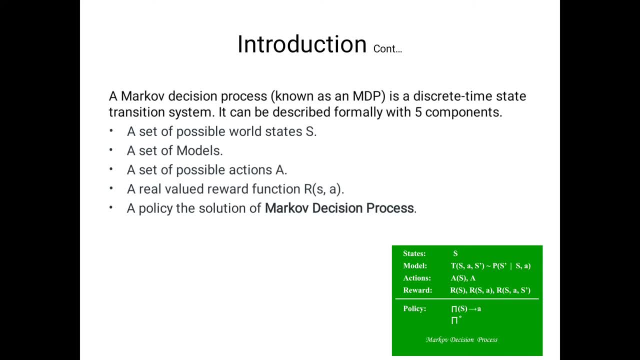 what is the state of action, and what is the state of action, and what is the state of action and what is the probability for getting the solution. that's why, therefore, here we will mention the probability of s dash. okay, so here the probability of s dash means. what is the probability? 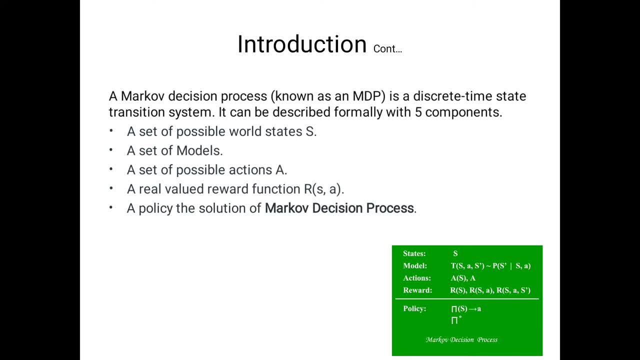 for to get the goal. okay, so that is dependent on the state. and action, okay. so here, what are the actions? here the actions are indicated by capital: a or a of s. a means simply the action, so a of s. the action is dependent on the particular state. here rewards: what is the meaning of r of s, r of s? 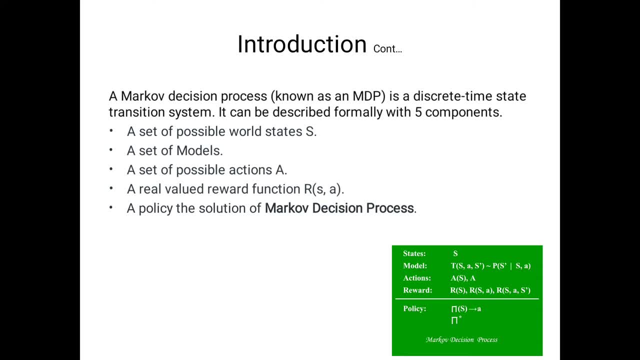 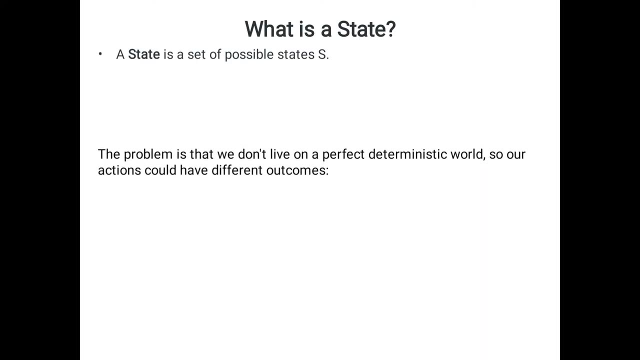 comma a r of s comma a comma s dash, we will see. okay, here the policy means simply the solution that is indicated by the phi. so we will discuss what is the meaning of phi of s implies a phi star, okay, so now let us start with the meaning of state. here the state is represented by capital s. 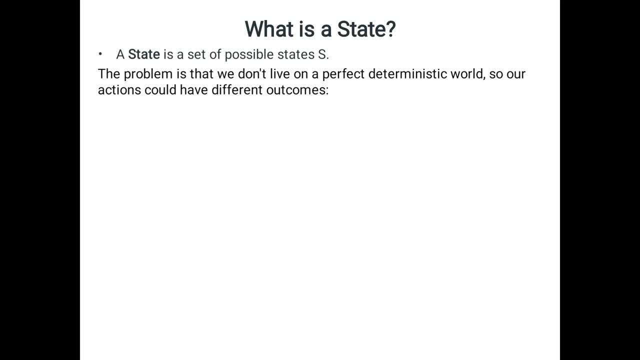 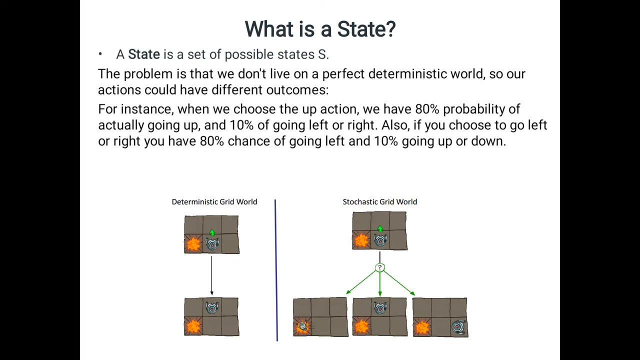 the problem is that we don't live on a perfect deterministic world. so far. okay, so far. actions could have different outcomes. okay, definitely. here we will find out the solution. here we will reach to the our expected goal only okay for that point of view. at each and every step we will find out the probability. so now, here i will mention two. 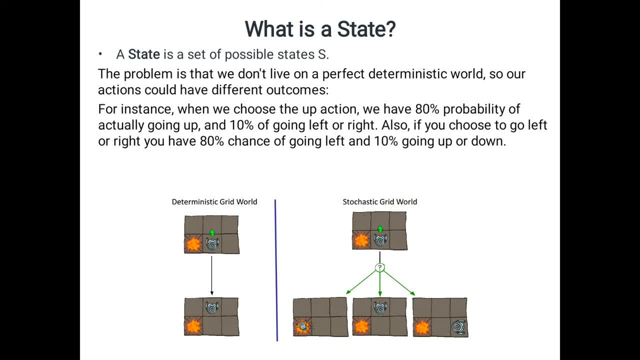 different types of walls: deterministic grid world and stochastic grid world. coming to the deterministic grid world, here the upper part determines: um, please observe, here the fire is available and the agent is available. suppose the agent moves to the left side? definitely it will be fired. so that's why here the options is: either move to 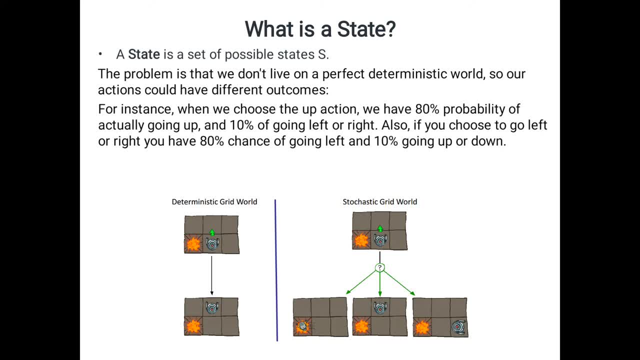 the upside or right side. those are the very good manner process, okay, so that's why here i will the agent move to the upside. okay, so suppose we will move to the right side. stochastic grid world. here what is the meaning of stochastic? it selects the answer, okay, so it depends on- totally depend on- the luck. so definitely here. 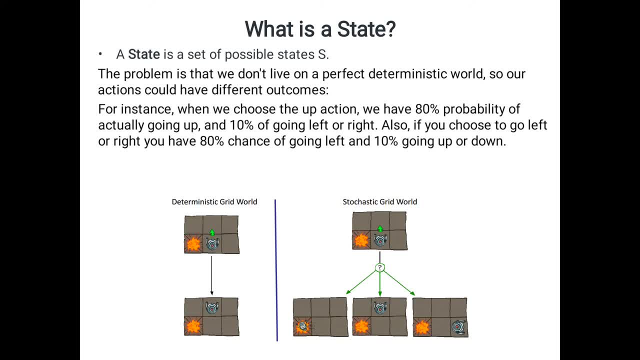 we have two or three options. what are the three options? so here the, that means in the stochastic grid world the agent move to the left side or upside or right side. okay, that's why here i will divide the three parts. so suppose the agent moves to the left side, then it will be fired, the agent. 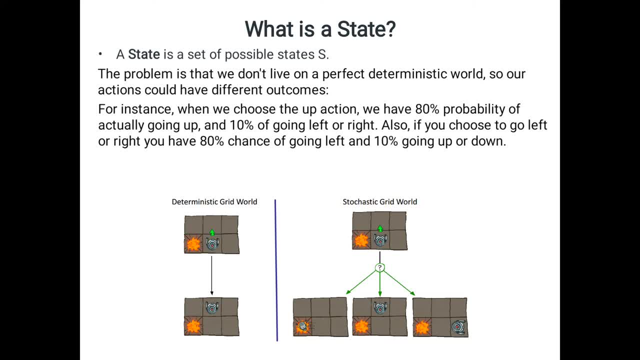 move to the upside, it will be safe, and the agent move to the right side, also, it is the safe. okay, this is the process. here each and every cell is represented by the state. okay, so here, with the help of state, with the help of action, here the action means either move to the left side or 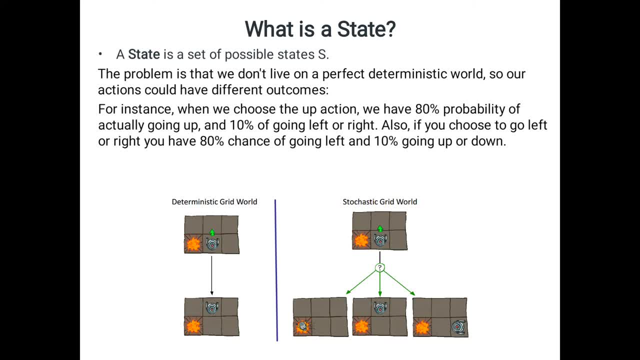 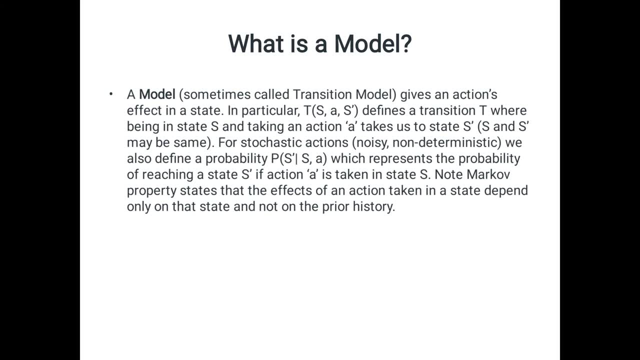 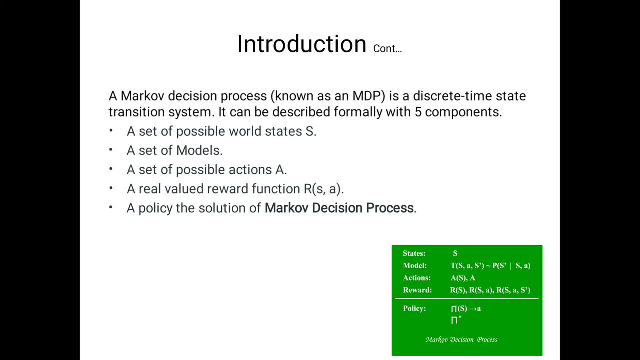 right side or upside. that is the meaning of actions. okay, so now we will see what is the meaning of model actually at the time of, you know please? so the this diagram. so here the model t of s comma, a comma s dash. so that's why the model. 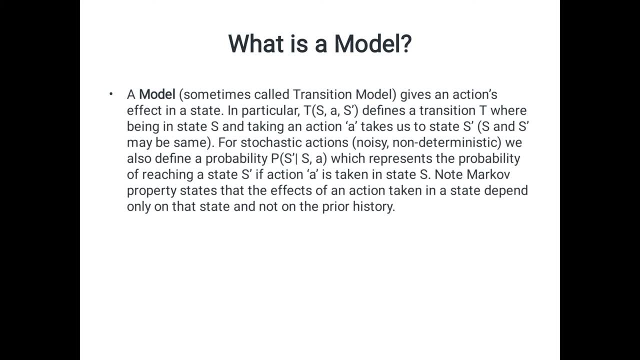 what is the meaning of t s a s dash? okay, here, t is the transition model. it takes the current state and current action and it produces the s dash. maybe s and s dash are the same here. okay, for the stochastic actions. what is the meaning of stochastic? either noisy or non-deterministic. 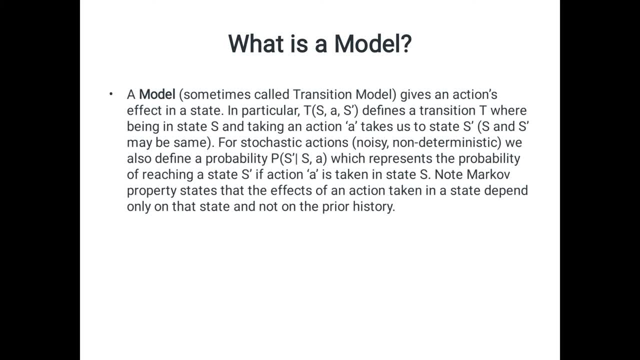 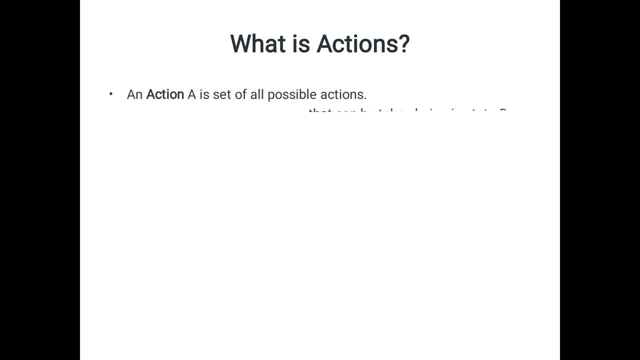 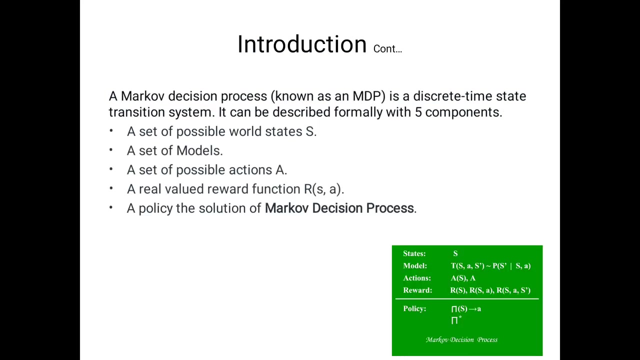 we also define the probability here. okay, what is the probability for getting the solution here? how to find out the probability? definitely, that is depending on the current state and current action. okay, so this is the meaning of model. now we will see the actions. what are the actions we will perform actually, here at the time of diagram, we will see the representations of. 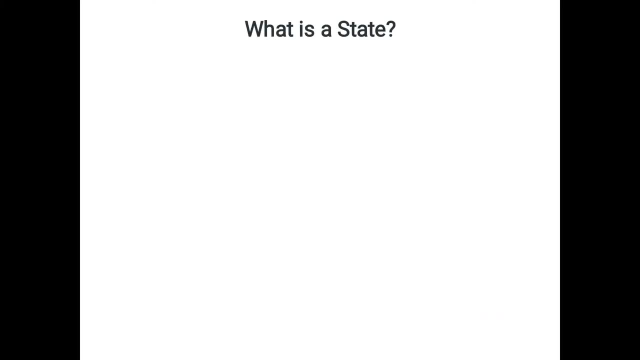 actions are a of s and a. what is the meaning of a here? what is the meaning of a of s here? simply, the a means set of all the possible actions. a of s means so the particular action is dependent on the particular state. okay, so now we will see the rewards in the reward. 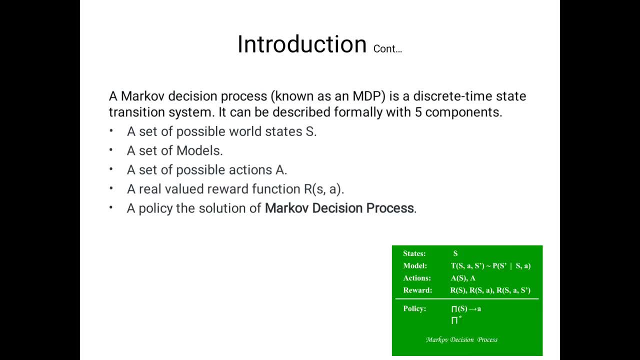 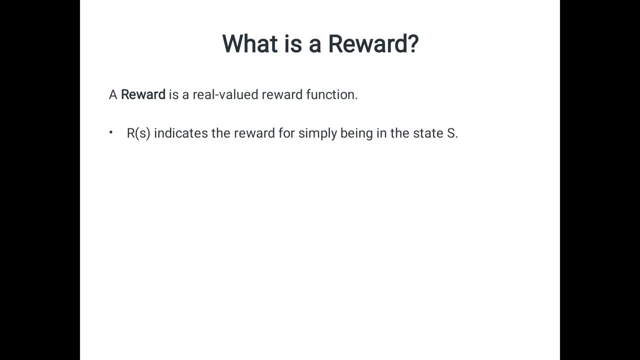 point of view. also, we will see the three different types of rewards: or of yes, or of s comma a r of s comma a common yes. okay, so we will see what is the meaning of R of yes. what is the meaning of our afternoon? is a-s comma, a comma s? that should he actually hear. 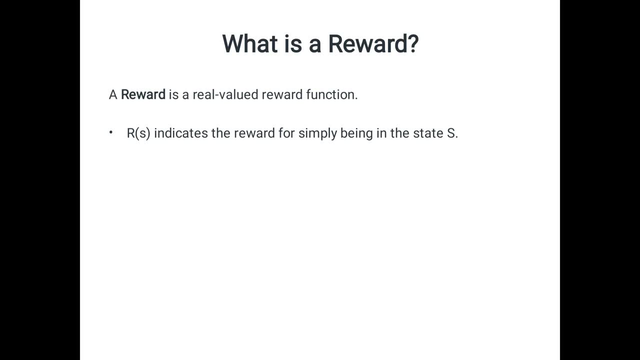 the reward is a real valued reward function. so our office indicates the reward for simply being in the e falta diva state. yes, here r of s comma a means here the reward is dependent on the action. okay, that's the reward for being in a state. yes, and taking an action. small a in the terms of r of s comma. 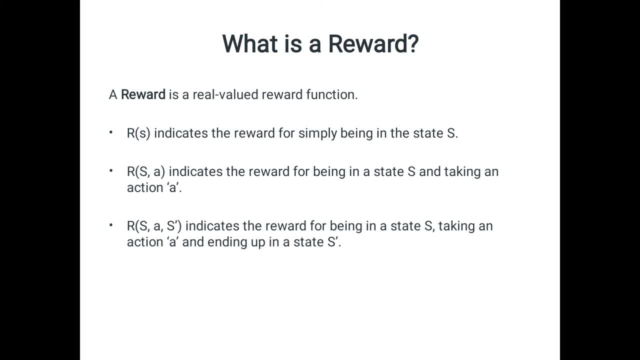 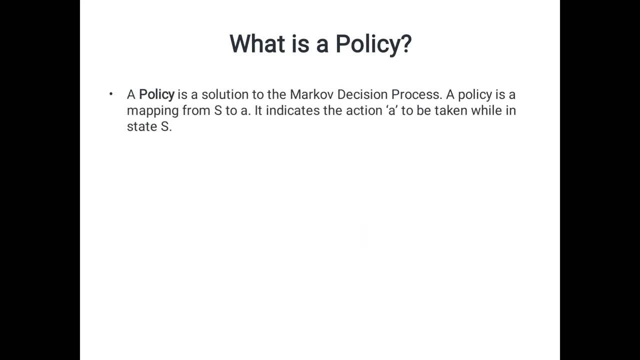 s dash. so here r of s comma a comma s dash indicates the reward for being in a state, capital s taking the action, small a and the expected state ending up in the state s dash. that is the meaning of reward here. finally, what is the meaning of policy? policy means simply the 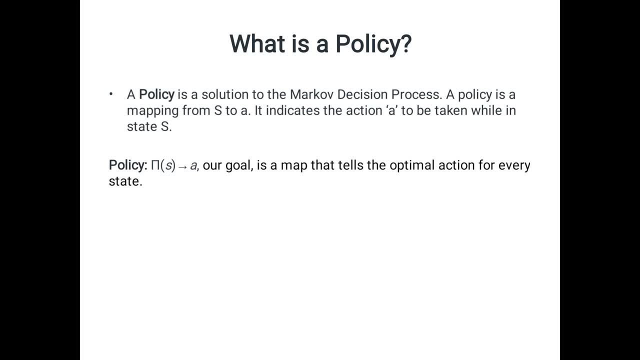 solution for the marco decision process. actually, here the policy is a mapping from s to a, so definitely depending on the states and actions, then only we will find out the solution. here the policy is denoted by the phi. here what is the meaning of phi and what is the meaning of? 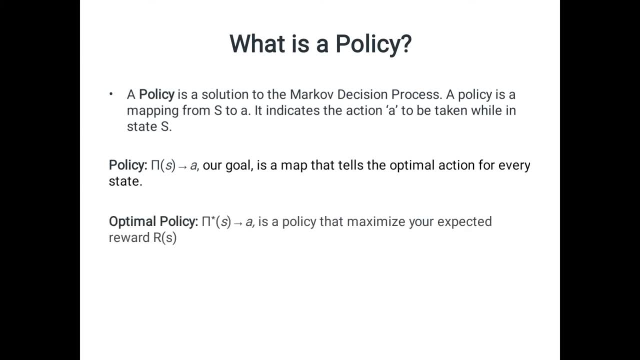 phi star. phi star means simply the policy, phi star means optimal policy. okay, so that's why here we will assumed as two different types: phi of s implies a phi star of s implies a here. phi of s implies a means, simply the goal. okay, actually it is a map that 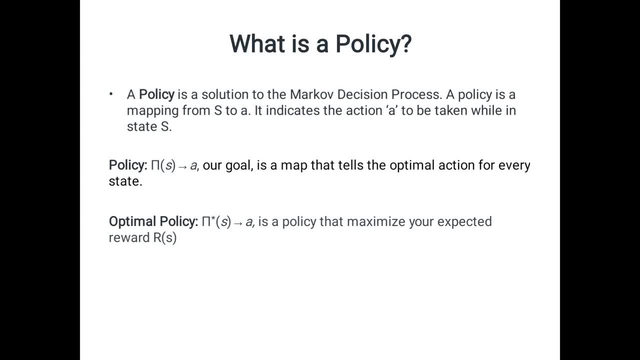 tells the optimal action for every state, but at the same time, the optimal policy says that it is the optimal solution. okay, in it, here the maximize your expected reward. here we will definitely so. that is the optimal policy. so this is the information about the marco decision process.